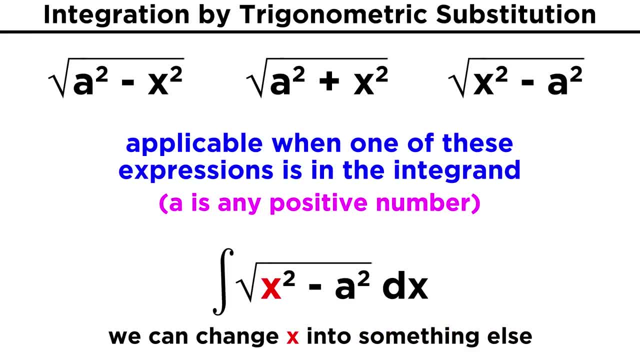 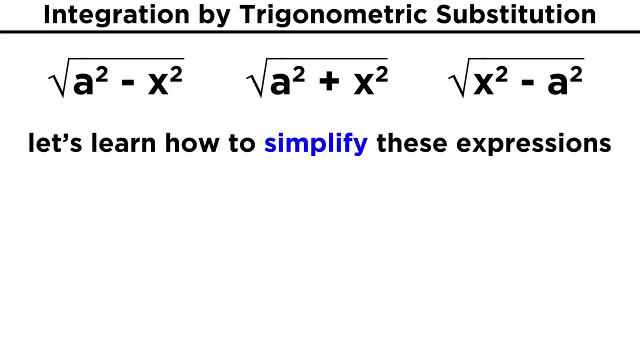 there is no term present to act as DU, But there is a different type of substitution we can use if we realize that we can change x into something else that will result in the ability to get rid of the radical. Let's first see what we can do to simplify these three expressions and then we will. 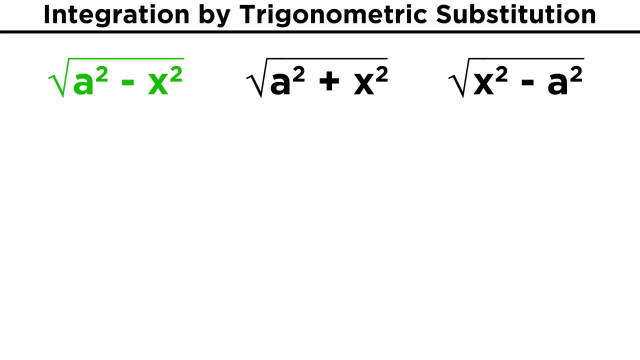 put that into the greater context of integration. Take this first example: with a squared minus x squared under the radical, Let's allow x to equal a sine theta. If we plug that in for x, the exponent distributes and we get a squared minus a squared sine. 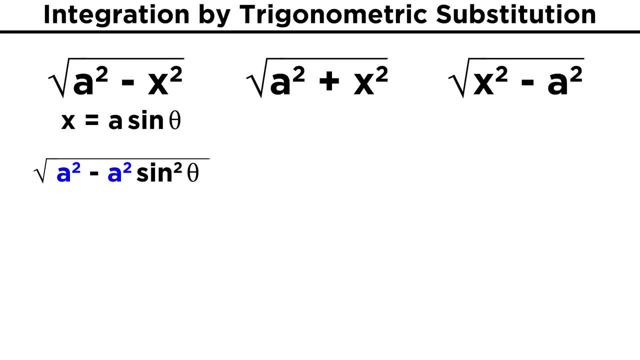 squared theta. Since we have a squared in both terms, let's factor that out to get a squared times the quantity one, One minus sine squared theta. We know from our Pythagorean identities that one minus sine squared theta is cosine squared theta. so let's make that change and we are left with a perfect square. 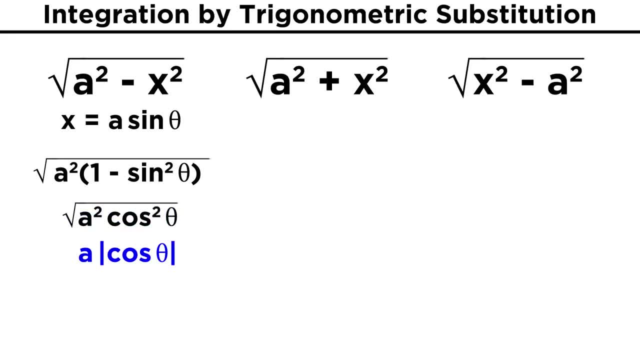 So let's take the square root and we are left with a times the absolute value of cosine theta. If we take the interval of theta as being between negative, half pi and half pi, we know cosine theta will be positive. so we can lose the absolute value and we are left with a cosine theta. 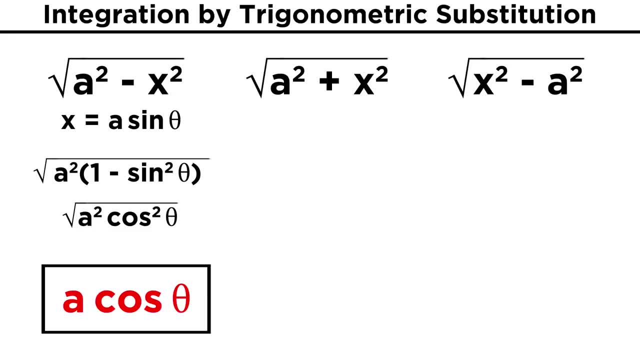 This is quite a bit simpler than what we started with, as you can see. Now let's look at the next expression: root a squared plus x squared. For this one, let's make x equal to a tangent theta. Just like the first example. we square it, factor out the a squared and we rectify that. 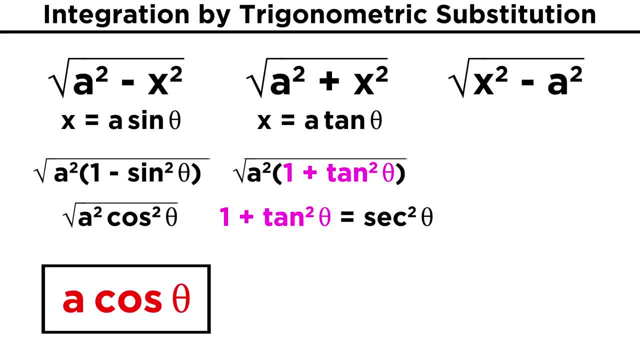 So we get a squared plus x squared. Now let's look at the next expression root: a squared plus x squared. We recognize that another Pythagorean identity is now applicable. One plus tangent squared is secant squared. So we apply that and then get rid of the square root to get a secant theta. 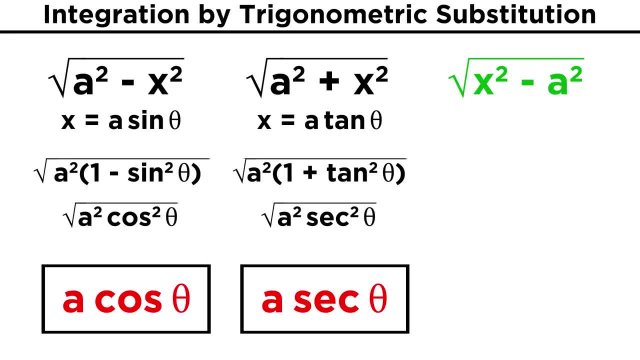 Again much nicer looking. And lastly, if we have root x squared minus a squared, we can change x into a secant theta. That gives us a squared, secant squared theta minus a squared. Again, we factor out the a squared and then realize that the same identity we used in 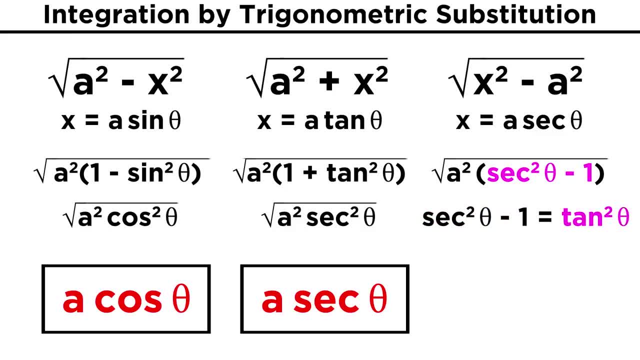 the previous example applies here, just the other way around. So we change secant squared minus one into tangent squared Again, the square root goes away and we have a tangent theta. So this is the first of three things we have to understand about integrating by trigonometric substitution. 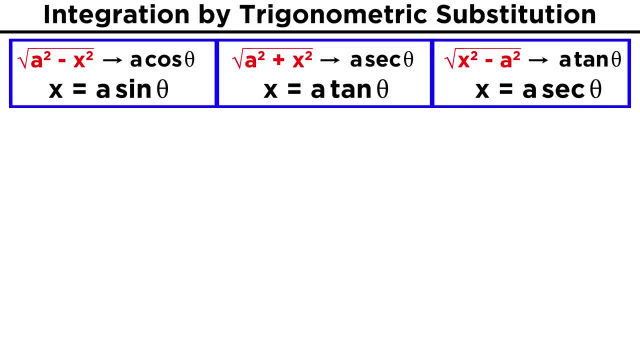 only be done when one of these three specific expressions is part of the integrand and there is a very specific substitution that must be done in each of the three cases: changing X into A sine theta, A tangent theta or A secant theta, depending on which expression. 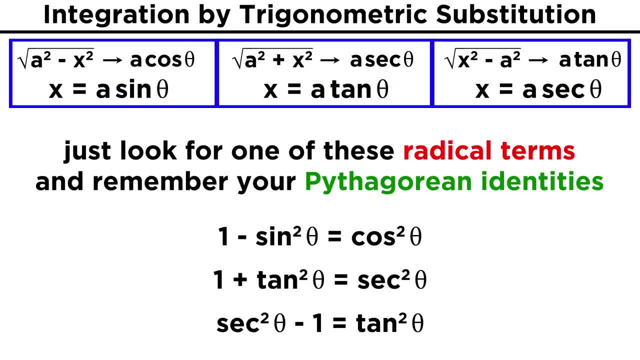 is present, But these conditions are not too hard to identify if we just remember that the goal is to get rid of the square roots and the Pythagorean identities relate sums and differences of squared things to squared things. However, this substitution and simplification is only the first part of the technique. 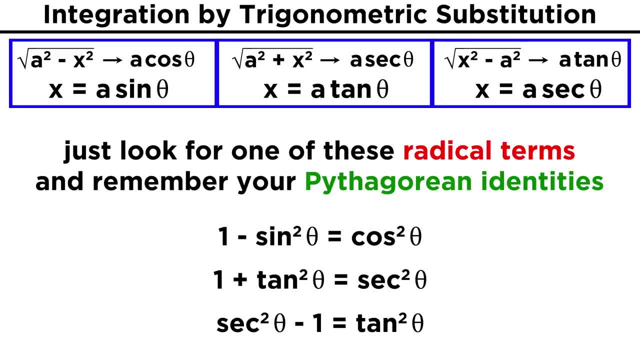 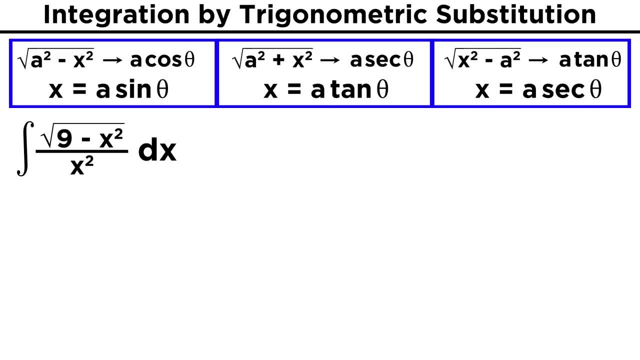 To see what else there is to it. let's look at a specific example to see why this substitution becomes useful. Take something like the integral of root nine minus X squared over X squared DX. We look at this radical term and we see that it is one of the expressions that qualify. 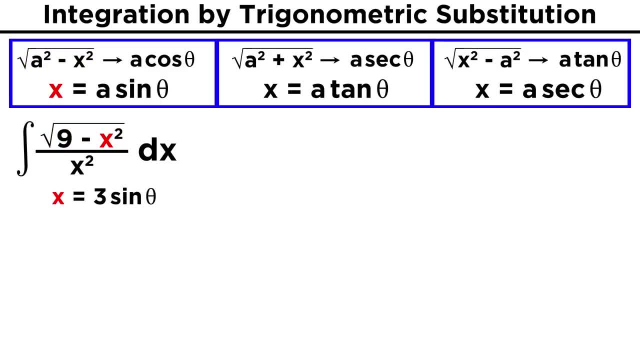 this for trig substitution. In this particular case we are going to change X into A sine theta and for this example, if the term starts with nine, nine must be A squared, so A will be three. That means X must specifically be substituted with three sine theta, and by the steps we 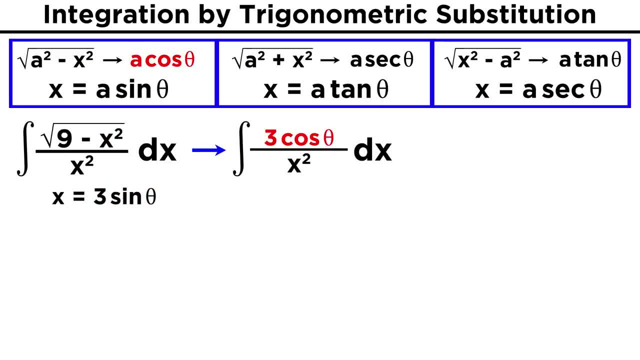 already discussed, this whole thing becomes three sine theta. So we can see that the integral of root nine minus X squared is three sine theta. So we can see that the integral of root nine minus X squared is three sine theta. This whole term will become three cosine theta. 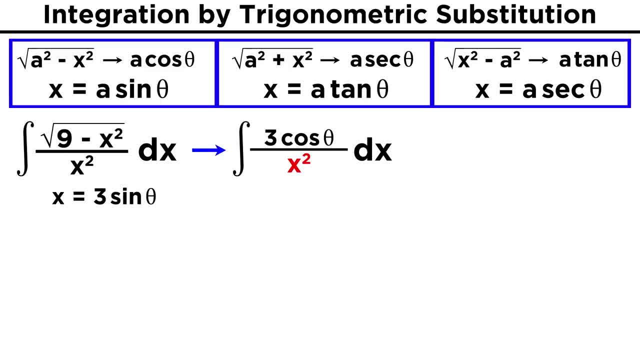 But that's not the only X in the integrand This X squared term in the denominator will become three sine theta quantity squared, or nine sine squared theta. Now here's the next thing we must keep in mind with this approach. This integral was in terms of X, so there is still a DX here. 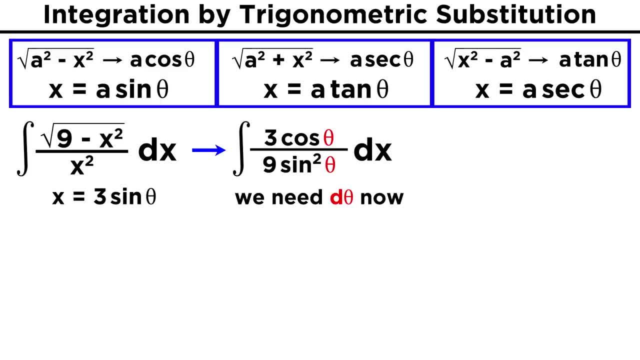 But if we changed everything to be in terms of theta, then this must also be in terms of theta. This must become D theta, otherwise we can't integrate with respect to theta. So what is DX in terms of theta? Well, if X is three sine theta, then DX over D theta must be its derivative, with respect. 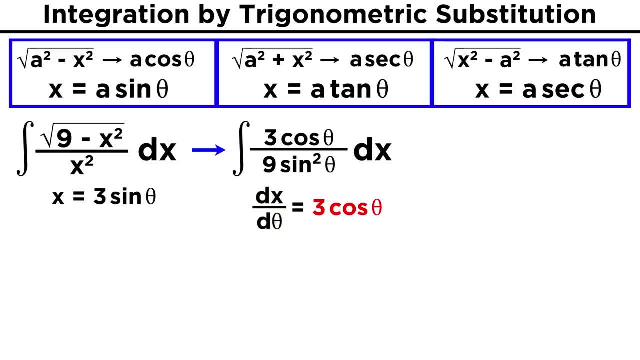 to theta. The derivative of three sine theta is three cosine theta. Then we bring D theta up here and that allows us to change DX into three cosine theta, D theta. Now everything is in terms of theta and we are ready to integrate. 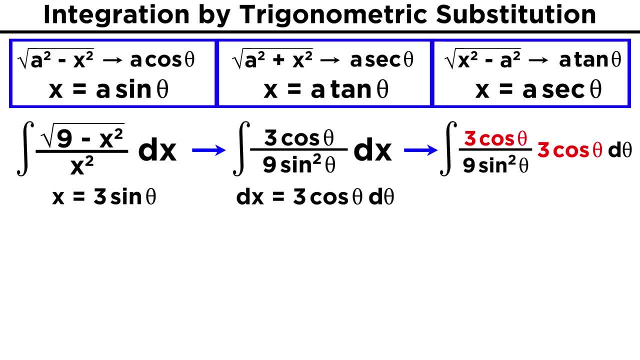 We can multiply this first three cosine theta by this new three cosine theta to get nine cosine squared theta. The nines cancel and we are left with cosine squared over sine squared, which is cotangent squared. Cotangent squared is not a common integral, so let's try to change the way it is expressed. 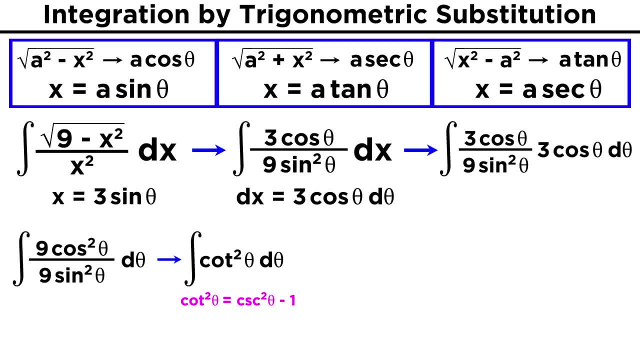 using some identity. The easiest one would be the identity that tells us that cotangent squared is the same as cosecant squared minus one. So we make that change, which is advantageous because cosecant squared can be directly integrated, Since the derivative of cotangent is negative. cosecant squared- cosecant squared- theta integrates. 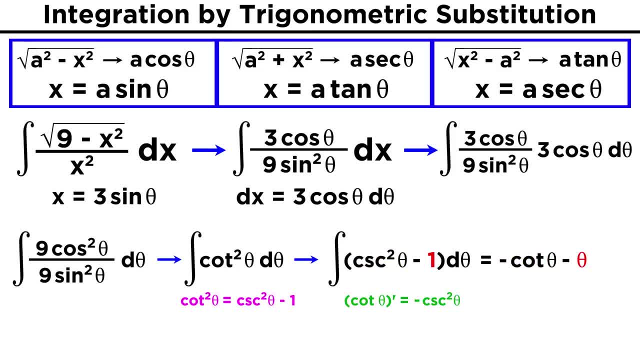 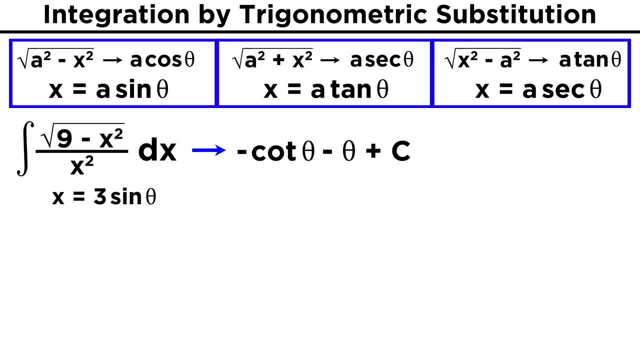 to become negative cotangent theta, And the one must be negative So we can integrate. It becomes theta, so we have negative cotangent theta, minus theta and then plus C, as usual. So the integration was successful, but unfortunately we still are not quite done. 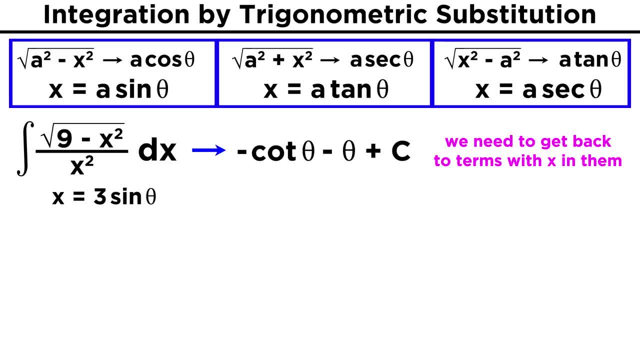 We wanted to integrate in terms of X, but we integrated in terms of theta. Not to worry, we can convert back to a form with X's in it without too much trouble. Let's just make a triangle. Let's make a triangle that looks like it is in the first quadrant and label the angle. 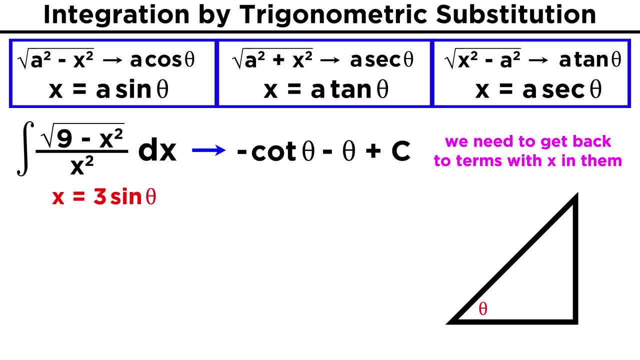 theta. Now, according to our original substitution for X, what will these sides be? Well, if X was equal to three sine theta, then sine theta must be equal to X over three. Sine theta is opposite over hypotenuse. so, according to our own substitution, this vertical: 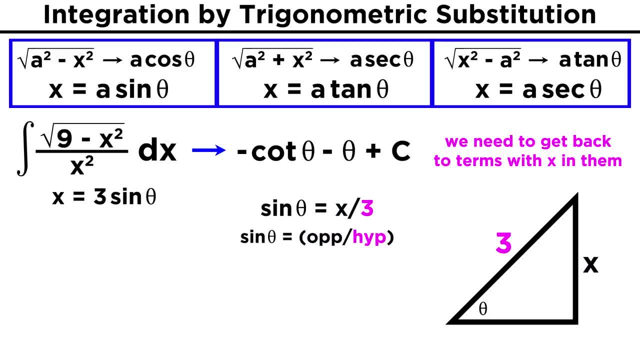 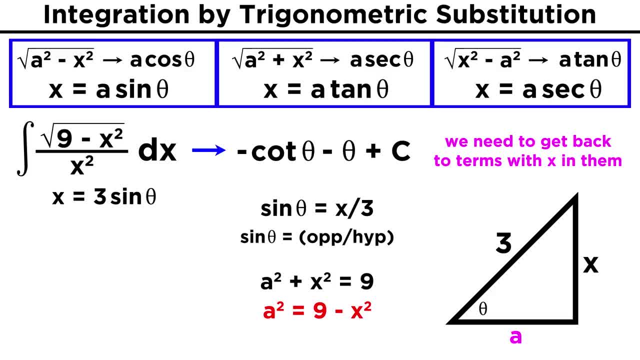 X squared must equal nine. so we subtract to get nine minus X squared and then take the square root to get root nine minus X squared. Now, with all of these sides labeled, we can express terms with theta in terms of X instead. 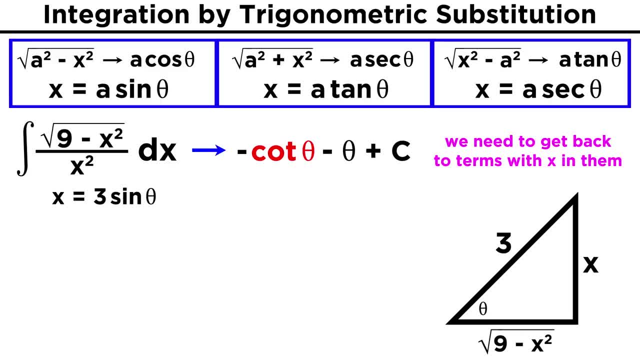 We have a cotangent theta And we know that cotangent is the reciprocal of tangent. If tangent is opposite over adjacent, cotangent is therefore adjacent over opposite, And in this case that is root nine minus X squared over X. So negative cotangent theta becomes negative, this expression we just found, and then for. 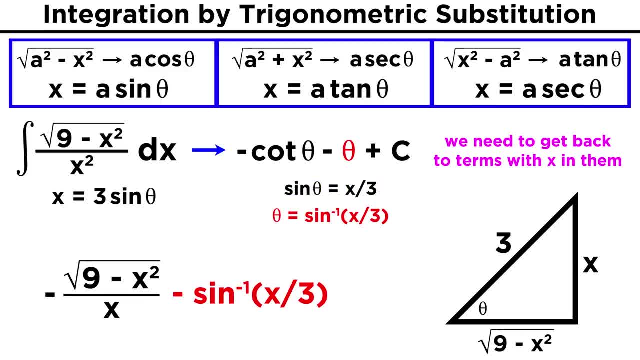 theta. if sine theta is X over three, then theta must be the inverse sine of X over three, of x over three. Then we include plus C and that will be our answer. So that may seem quite involved, but remember that we really just did three things. 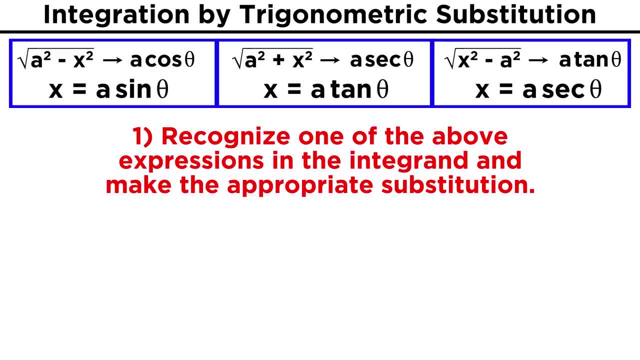 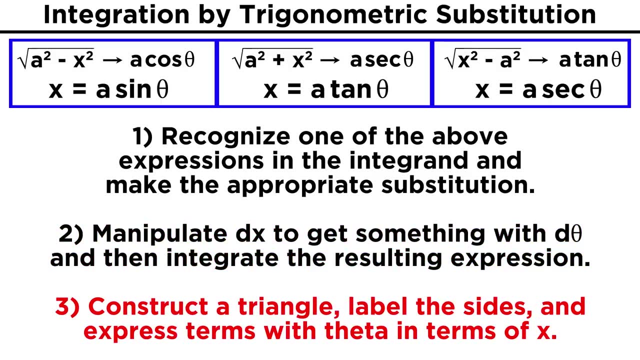 First we recognized one of the three expressions that allow for trig substitution and we made the substitution. Then we manipulated dx to get an expression with d theta in it, which allowed us to integrate by whatever means now possible. Then, to get our answer back in terms of x, we constructed a triangle and labeled everything. 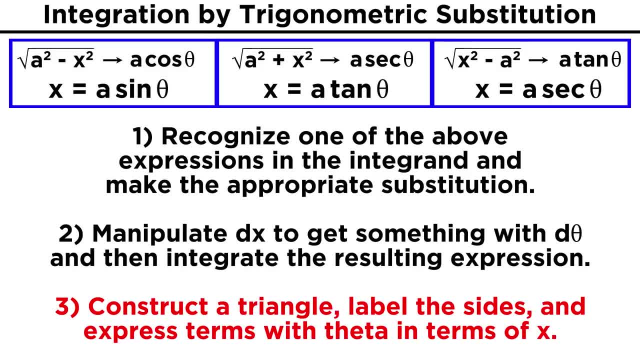 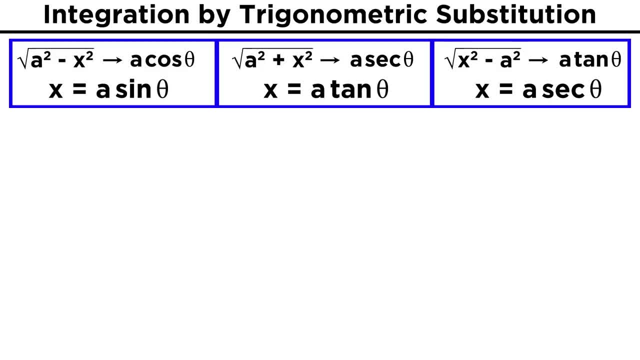 in terms of x, so that we could express our answer in terms of x. Don't worry, this will get easier over time. Let's try one more to help things sink in. How about the integral of one over the quantity x squared times root x squared plus four? 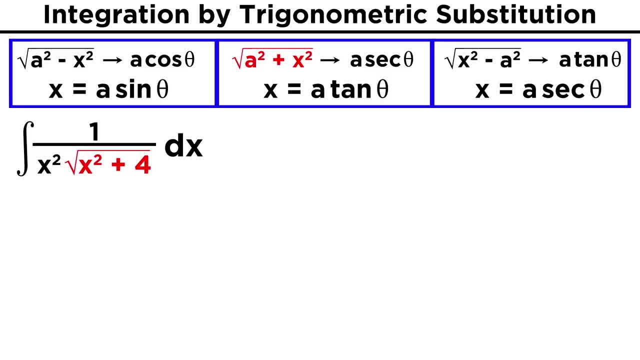 dx. The first part is easy. we just recognize that this radical expression is one of the three that can be simplified by trig substitution and we recall that with this particular expression we allow x to be substituted by A tangent theta. In this case, if A squared is four, then A is two, so we will allow x to become two tangent. 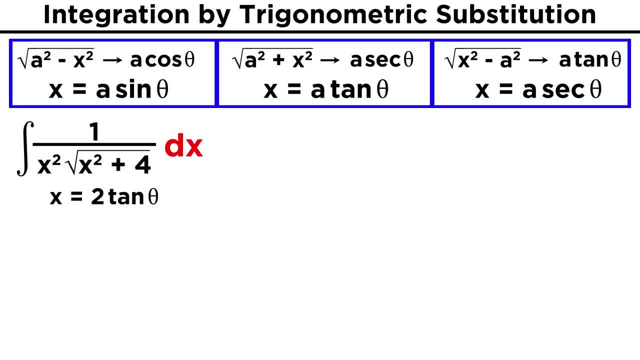 theta. Let's go ahead and take care of dx while we are at it. Finding dx over d theta will require taking the derivative of tangent, which is secant squared, And then we bring d theta up here to get two secant squared: theta, d theta. 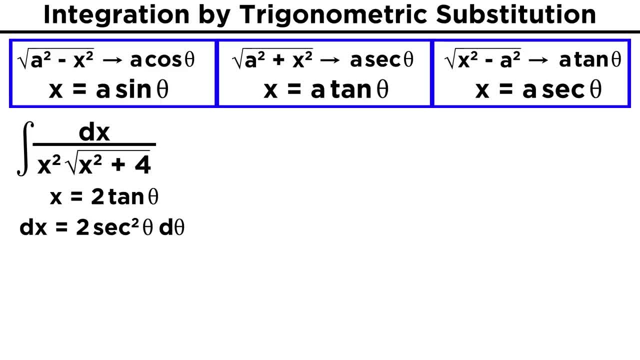 So we go ahead and transform our integral, putting dx up here in the numerator to make things simpler, and we get two secant squared theta d theta over four tangent squared theta times two secant theta. Now let's look at the integral. Now substitution is complete and it's time to perform the integration. 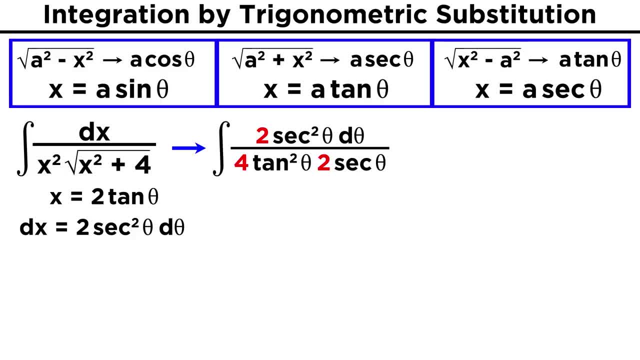 First, we can simplify a little bit. The numbers simplify to one fourth, so let's take that out of the integral to make things simpler. One of the secants will cancel and we are left with secant theta over tangent squared theta d theta. 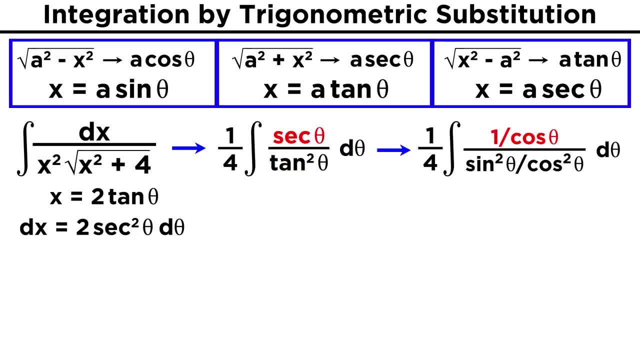 Let's change secant to one over cosine and tangent squared to sine, squared over cosine squared. Then we can multiply the numerator by the reciprocal of the denominator. One cosine cancels and we are left with cosine theta over sine squared, theta d theta. 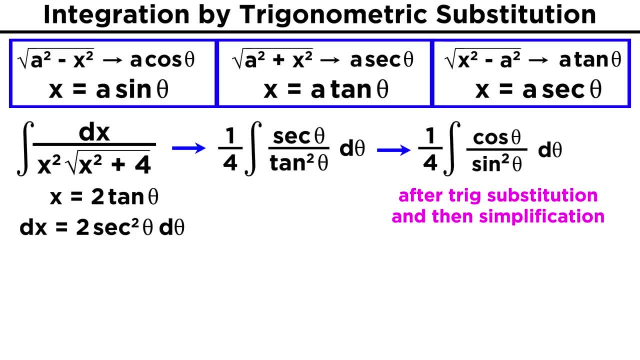 Now, once we are here, after performing the trig substitution and simplifying as much as possible, we ought to have something that can be integrated, but it may require another one of our techniques. In this case, we can do another substitution. Let's say that u equals sine theta. 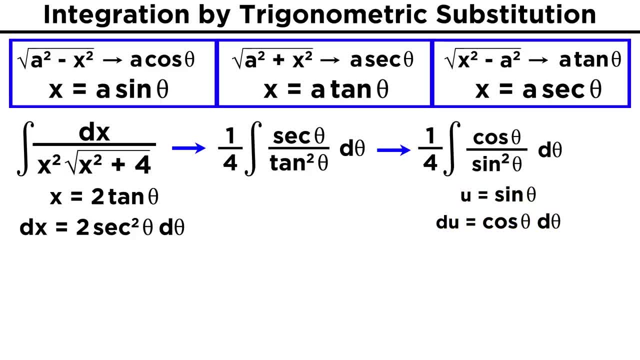 Then du will be cosine theta, d theta. That ends up coming in handy, because this integral then becomes du over u squared. This is finally something that we can integrate directly. U to the negative two becomes u to the negative, one over negative one or negative one over. 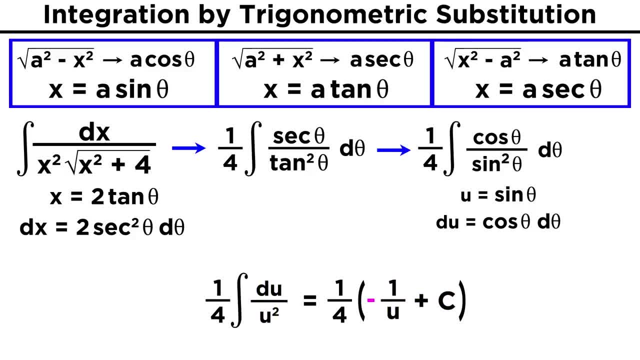 u plus c. We take the negative out here to get the integral. Then we integrate the integral To join the one. fourth, change u back into sine theta and we are left with negative one over four, sine theta plus c, If we prefer, one over sine can become cosecant. so let's change this to negative cosecant. 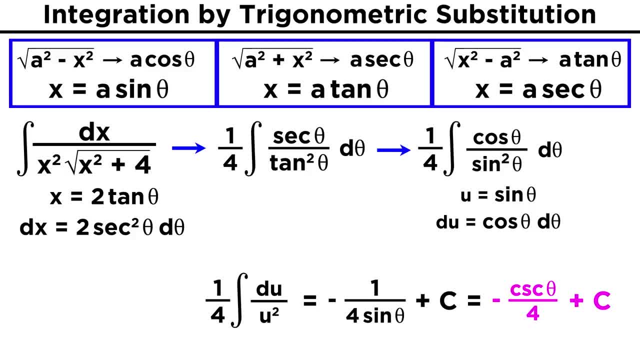 theta over four plus c. So we got from u back to theta. but remember we now have to go from theta back to x. so let's make our triangle, We place theta And then we consult the original substitution we made, which was x equals two tangent theta. 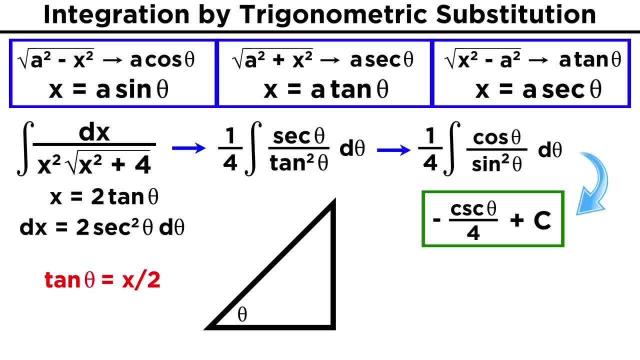 Therefore tangent theta equals x over two. Tangent is opposite over adjacent, so this opposite leg must be x and this adjacent leg must be two. Then by the Pythagorean theorem, the hypotenuse must be root x squared plus four. 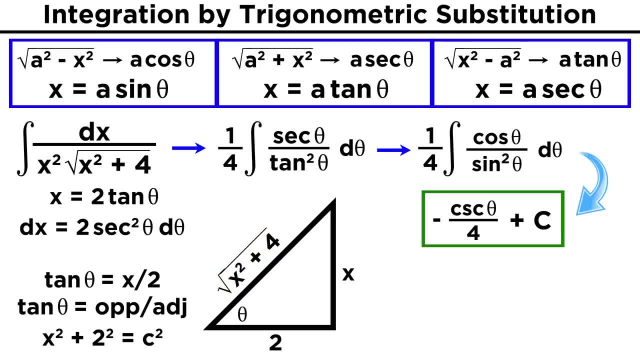 Now we have our triangle set up, so let's check back with our answer to see what the answer is. Let's go back to the previous example. Let's see what needs to be done. We have a cosecant theta term in there, and if sine is opposite over hypotenuse, then 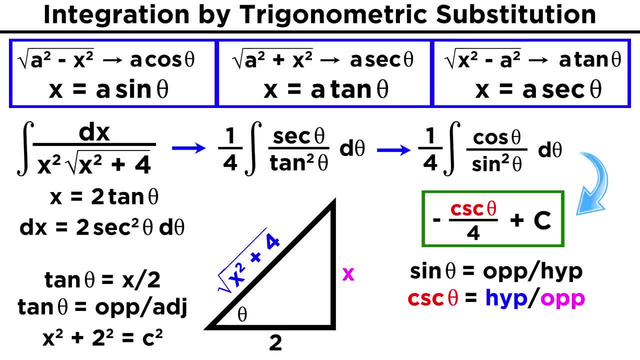 cosecant is hypotenuse over opposite. In this case that will be root x squared plus four over x. So let's put that in there in the place of cosecant. theta, The denominator of the numerator can just be brought down to the denominator, and there 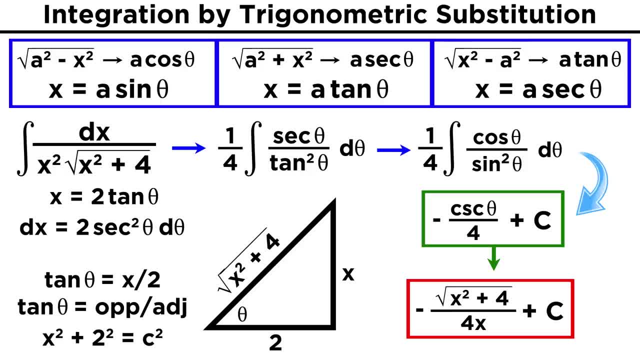 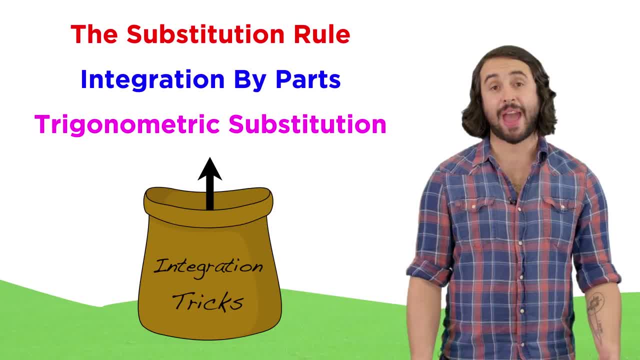 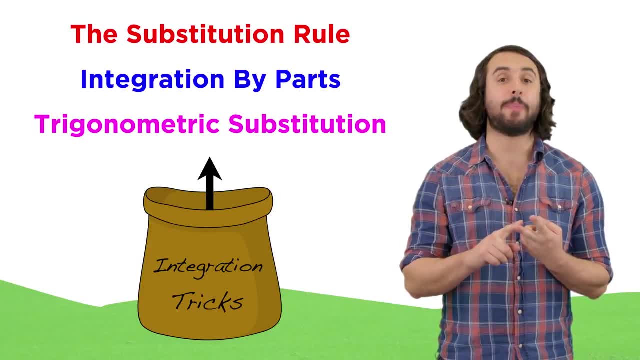 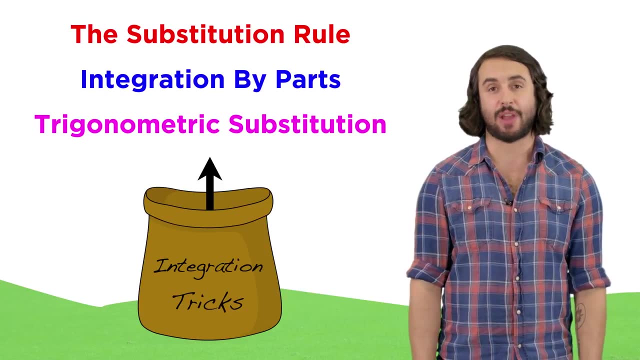 is our final answer: Five root x squared plus four over four x plus c. So with that, we now have three solid techniques in our bag of tricks, those being the substitution rule, integration by parts and trigonometric substitution. As we learned each of these techniques, it was quite obvious which strategy we would. 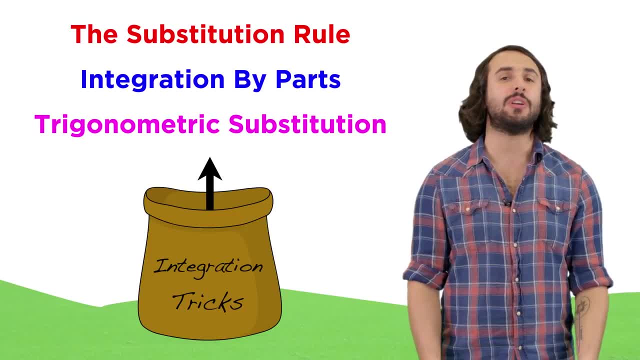 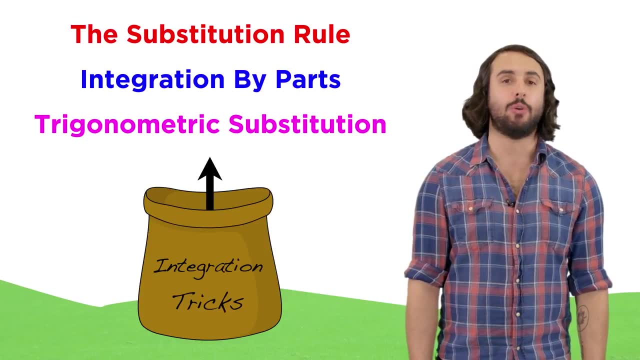 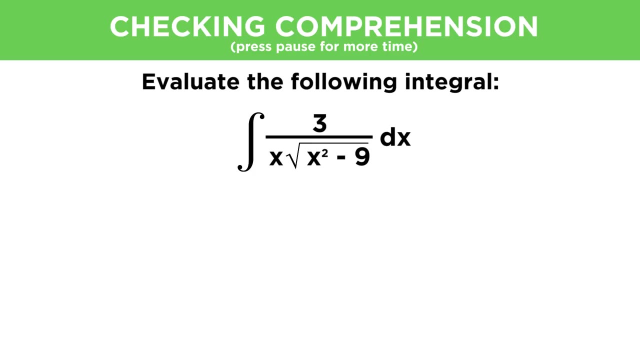 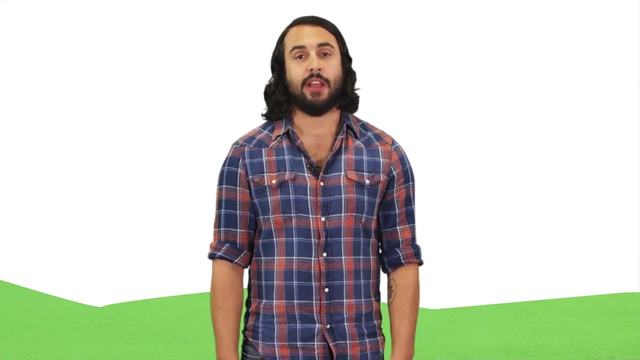 be applying in each example, but we also have to get used to looking at integrals without any context. In the next tutorial we will practice exactly that, but first let's check comprehension. Thanks for watching, guys. Subscribe to my channel for more tutorials. support me on Patreon so I can keep making.